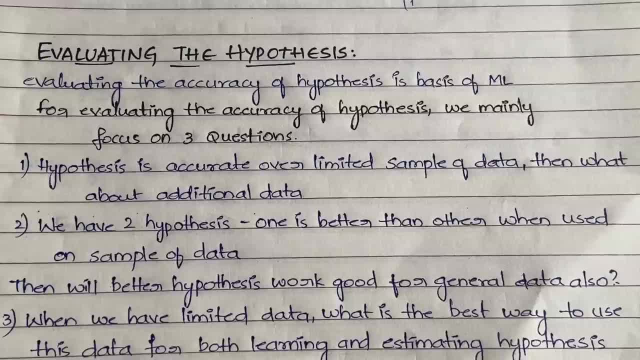 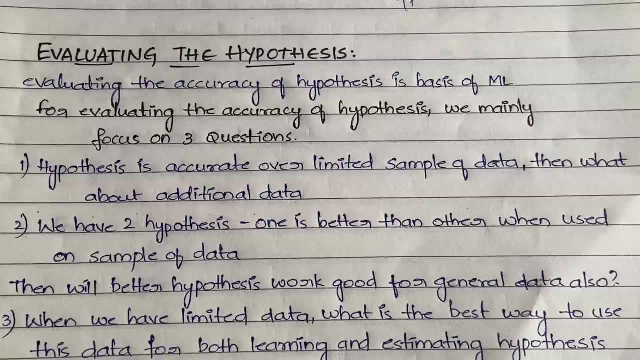 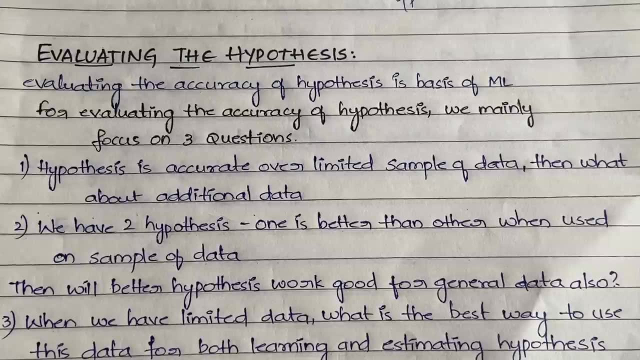 So that I can make videos according to your exam date and also your college name. you mention it in the comment section So that I can make according to your college syllabus. Okay, done, and now let's get started. So first, yeah, this concept is actually very, very, very boring and very you know, it's like you know you what is? you'll feel like: what is this like? 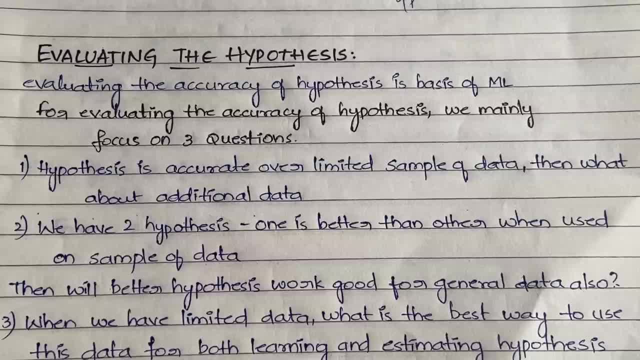 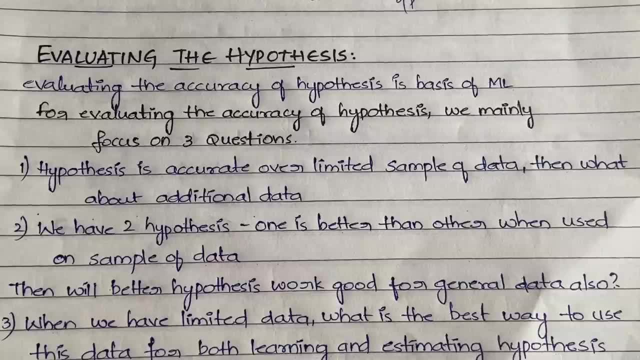 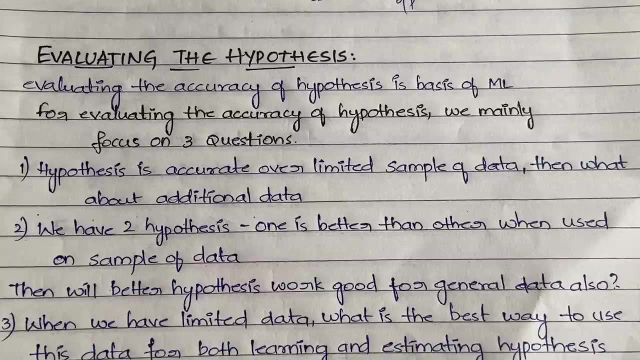 So, don't worry, Be patient. Pay 100% concentration towards the video. Watch the video till the end. Okay, so it is going to be more of theory. Okay, but you know theory and nothing relevant like that. It will be somewhat confusing, but I try to make it the best for you, So make sure you watch the video till the end. 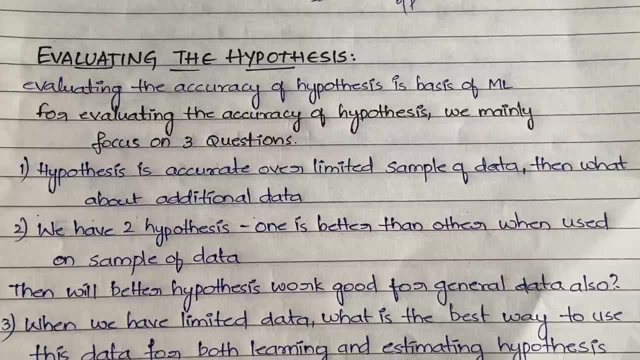 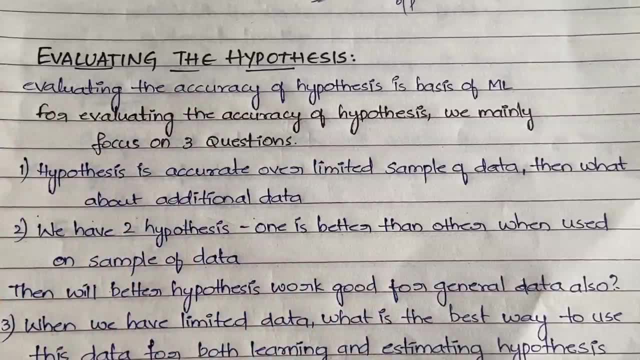 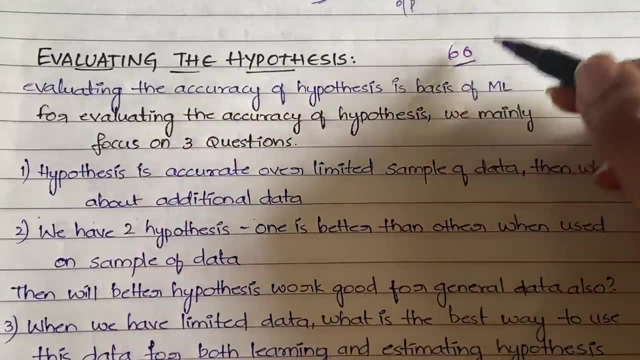 So first evaluating the hypothesis. So what do you mean by this? evaluating the hypothesis See to be simple. to be precise, evaluating the hypothesis is nothing. but suppose you have defined a hypothesis based on anything. Suppose in the class there are 60 students, In the class you are having 60 students and for this 60 students you have defined something like this: 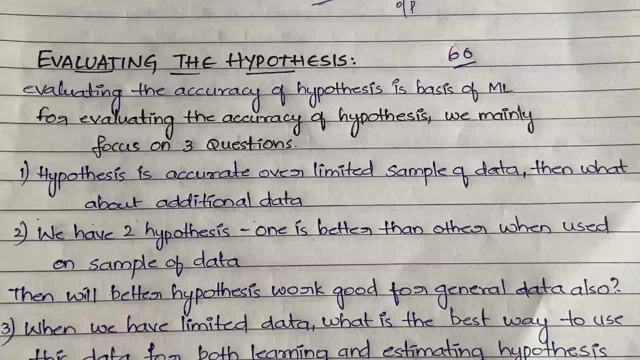 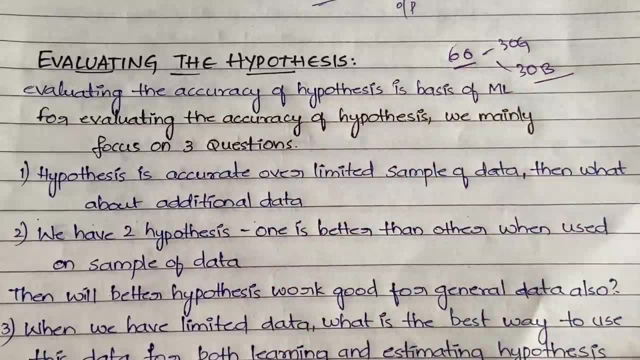 So, among 60 students, you have defined something like this: So, among 60 students, you came to a conclusion that there are 30 girls and 30 boys. You don't know, you don't have any evidence for this. You just came to a conclusion. 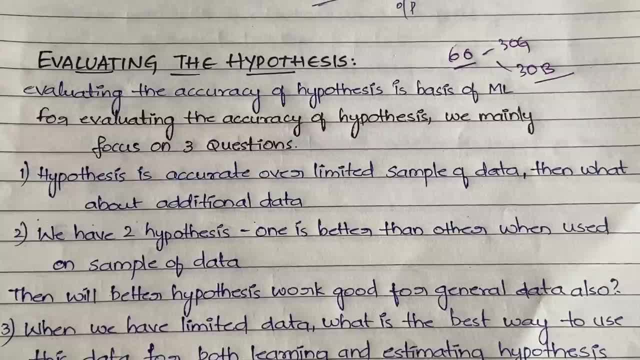 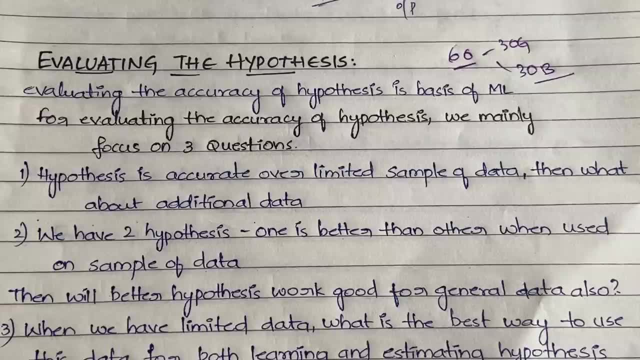 You've just assumed a hypothesis that there are 30 girls and 30 boys right Now. is this hypothesis true? If it is true, up to what extent it is true? What is the true percentage? Like it is 100% true, or it is 95% true, or it is 90% true, Like that? you need to evaluate the hypothesis. 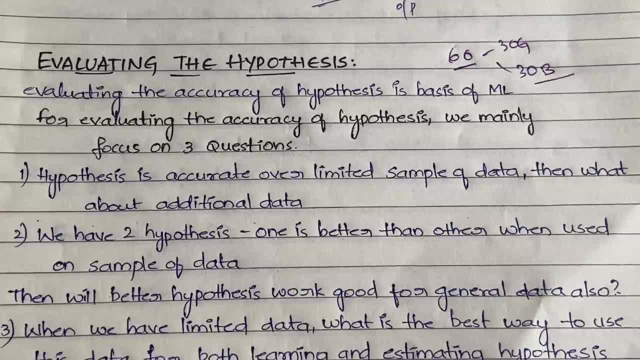 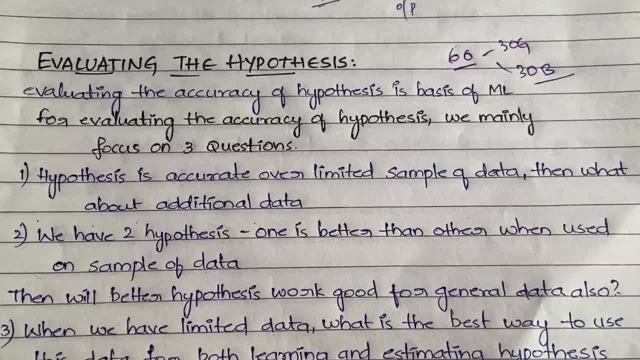 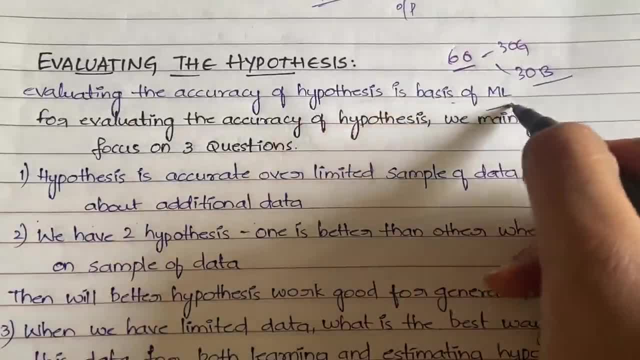 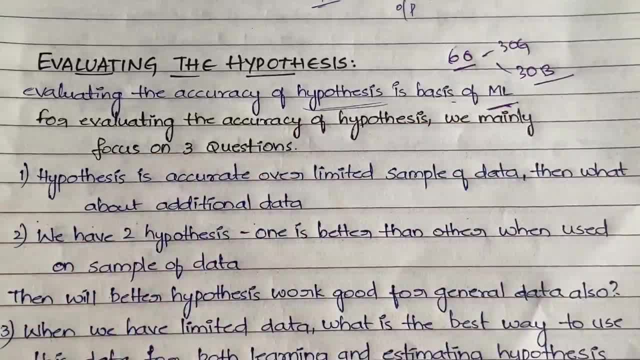 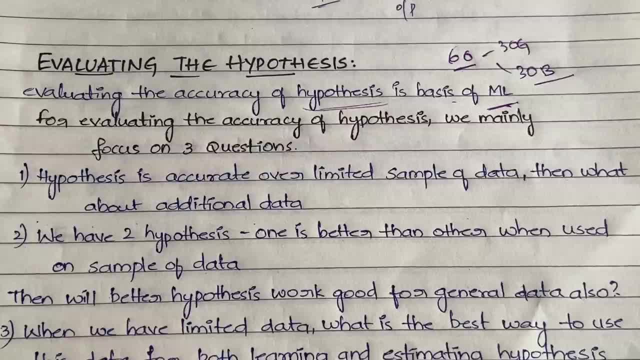 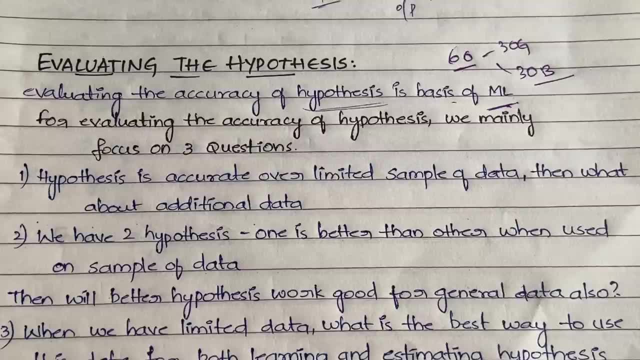 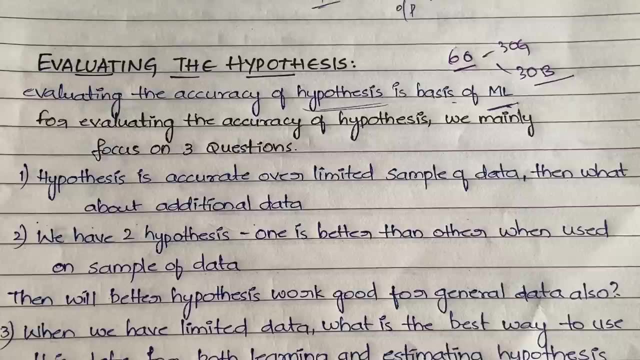 We have been seeing this word hypothesis right from the start of right from video 1, we have been listening to this word hypothesis right. So evaluation of hypothesis is also that important, because it is very important that we have to define or we have to give an efficient hypothesis which can cover all the types of 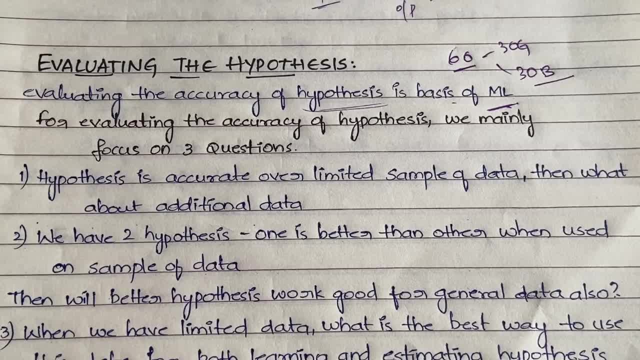 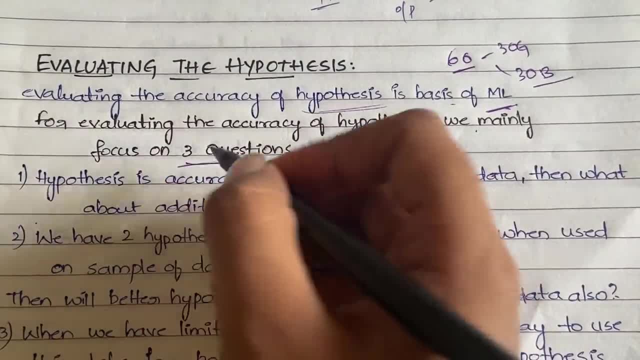 learning examples: okay, Done. So first, for evaluating the accuracy of the hypothesis, or for evaluating the hypothesis we, you have to mainly focus on 3 questions. okay, What are those 3 questions? I will tell you. You should mainly focus on 3 questions, and what are those are? 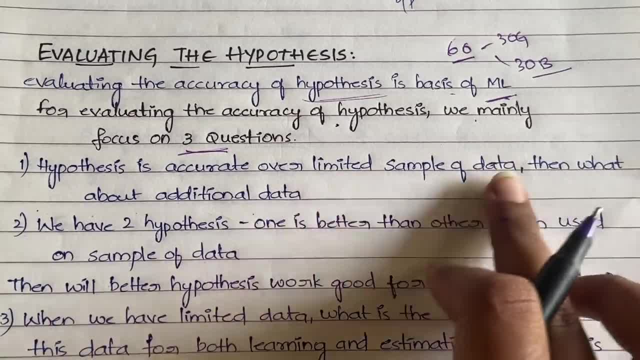 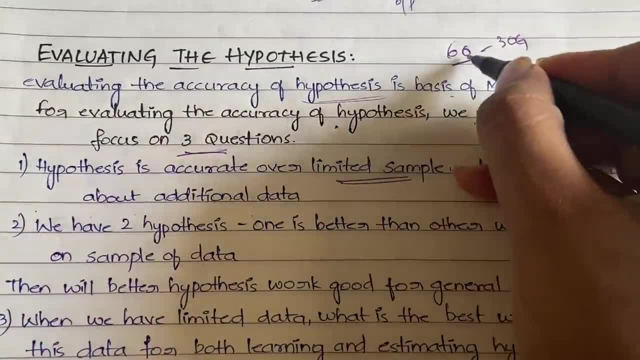 Hypothesis is accurate over limited sample of data, Then what about additional data? So you are defining a hypothesis over a limited sample of data. So, for example, here we have taken in a class of 60 students, we are taking 30 girls and 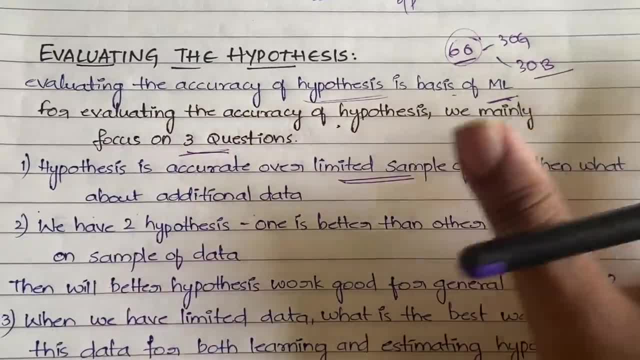 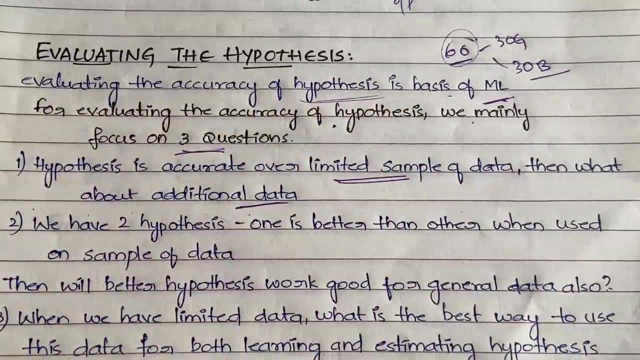 30 boys. okay, That is accurate, that is correct. whatever we have defined as accurate and correct. let us suppose Then: what about what happens? What happens when we add some additional data? Suppose some 10 or 20 or 30 newcomers join the class, then how do you classify them? 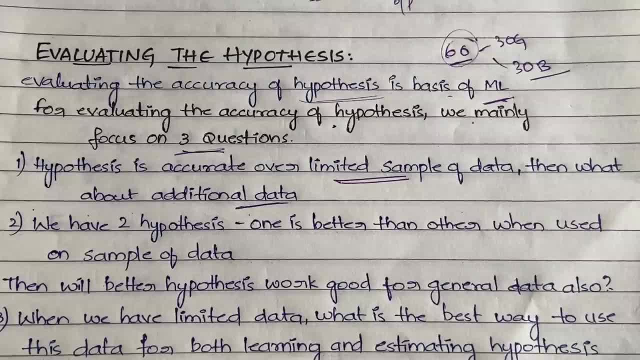 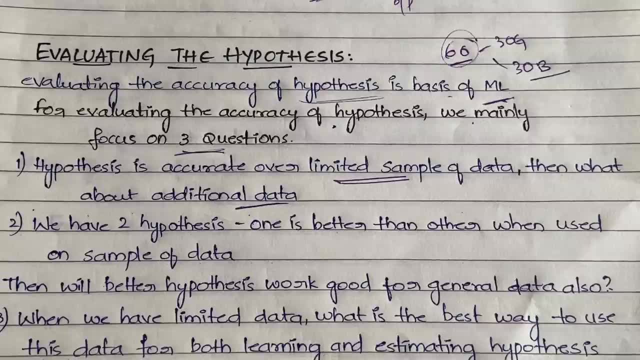 So previously, whatever hypothesis you have made is okay, correct for a particular sample of data, okay, But when some additional data is added? so what is the change in the accuracy right That you have to answer? And the second is we have 2 hypothesis. 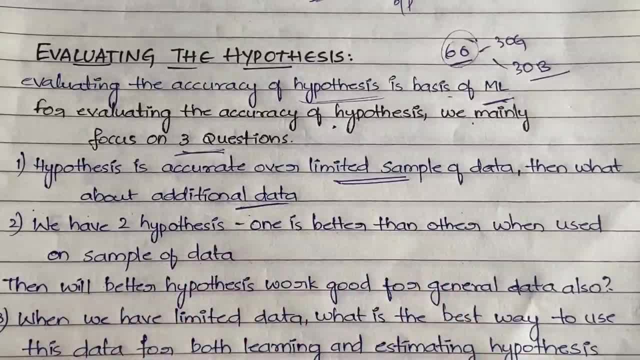 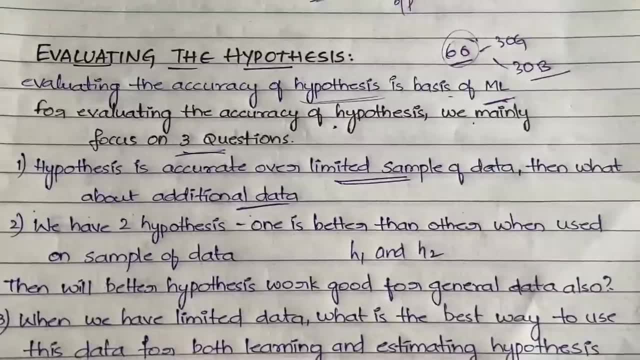 So among those 2 hypothesis, we came to a conclusion that one is better. right, So we have H1 and H2.. Then H2, let us take. So among H1 and H2, we came to a conclusion that H2 is better. okay, done. 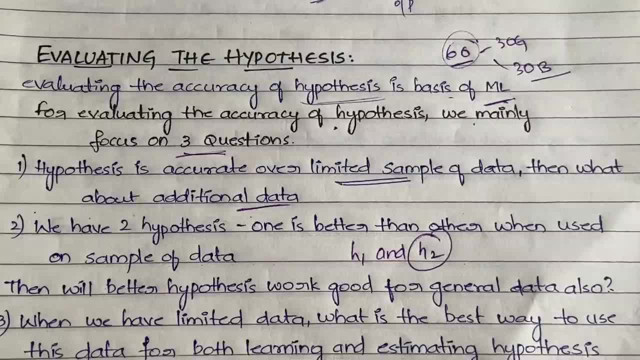 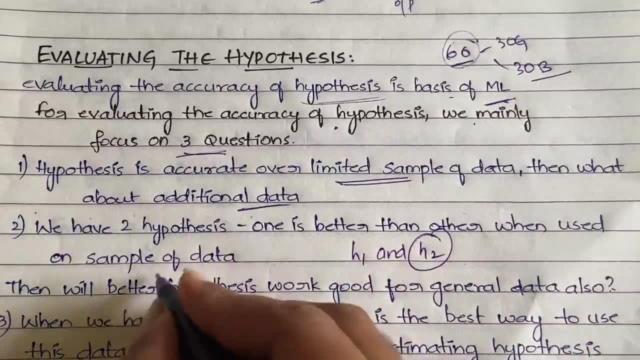 So we fixed, we have fixed on to H2, so we have fixed to use H2 as our final hypothesis And when you are getting this H2 as an efficient one or a better one, when you are testing it on sample of data, right, when you are using it on sample of data, you are finding. 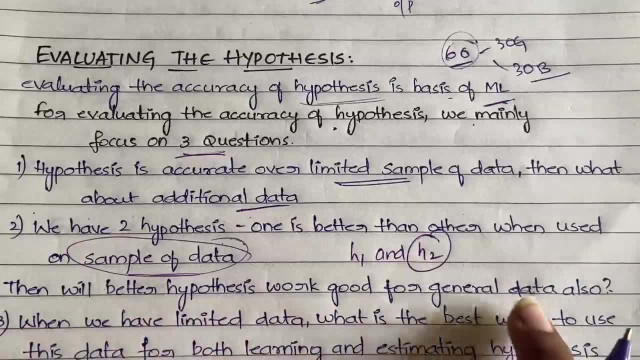 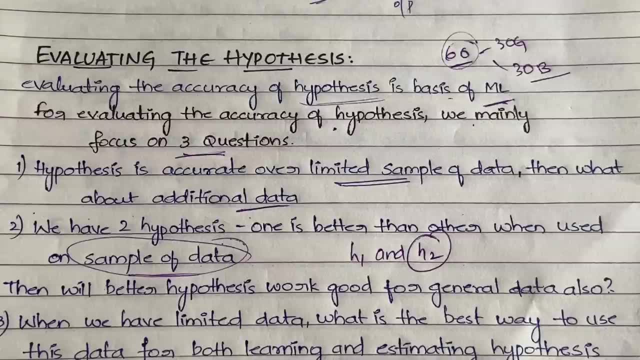 it to be better. But when you are using for general data, that is, when you are applying the entire data, Then will this H2 be better in that case. also, that is for some amount of data. okay, it is working good. 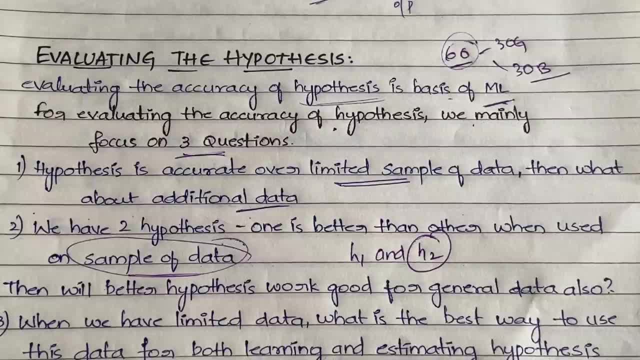 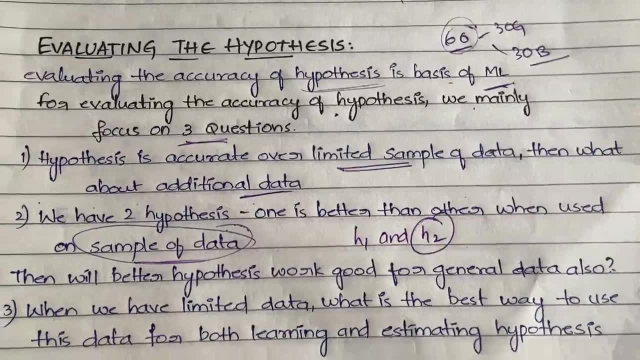 Then, what about the general data? what about entire data? will it work good, even for entire data? that also you need to question yourself. And the third is: when we have limited data, what is the best way to use this data for? 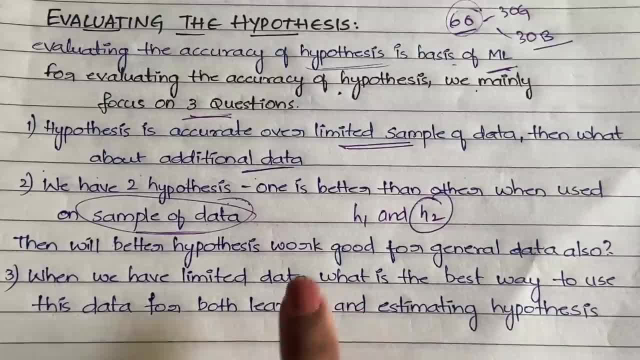 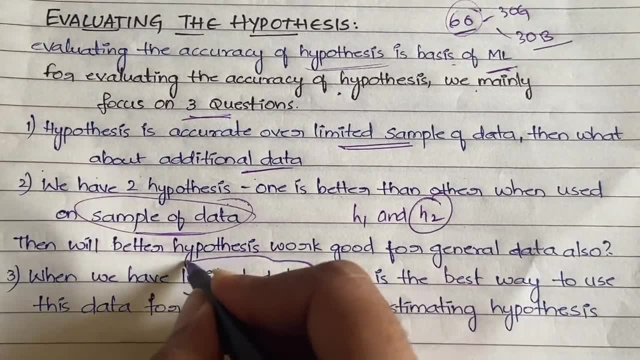 both learning and estimating the hypothesis. First is learning is also very important, right, the machine has to learn. So when you are having only limited data, when you are having only limited data, you need to know how to use, like how to, how you divide the data, how much percent of the 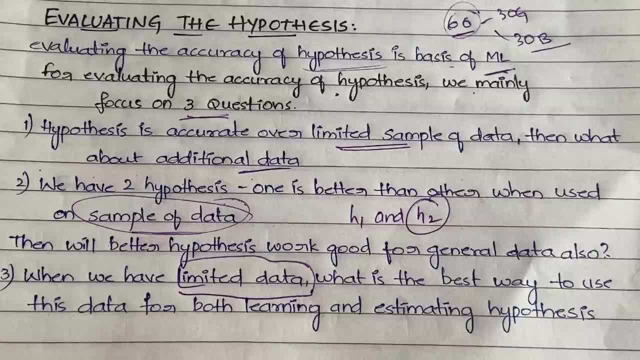 data you give for learning, how much percent of data you give for estimating the hypothesis. okay, So these are the three questions that are to be asked, or you need to focus on these three questions and you need to estimate the accuracy of the hypothesis based on these. 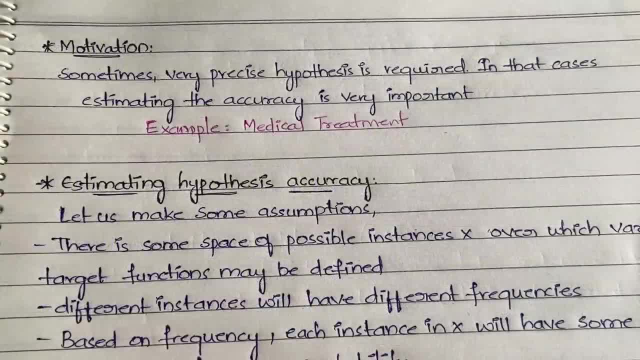 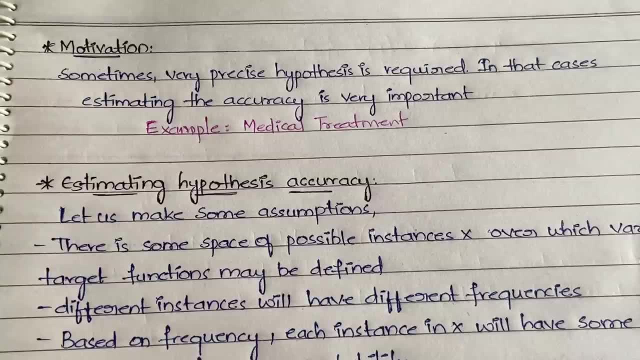 three questions. okay, done Now. what is the motivation? what is the motivation for estimating the hypothesis? why do you have to estimate the accuracy of the hypothesis? why do you have to check for the estimate accuracy of the hypothesis? hypothesis means sometimes, in some situations we will be having, we should have a very precise 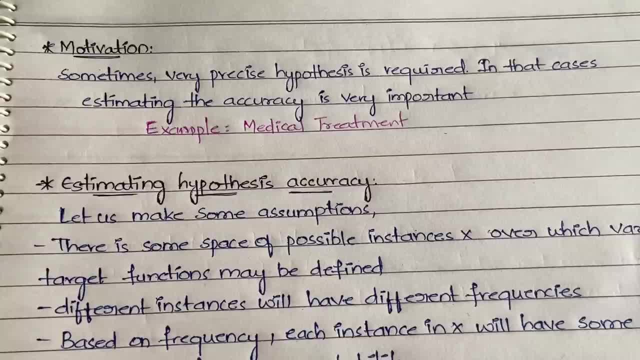 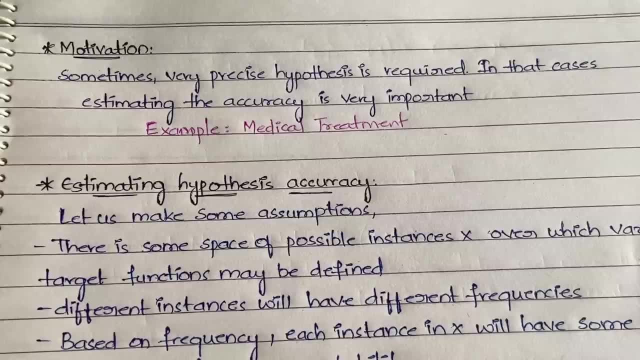 hypothesis right, a very precise, a very accurate, very sharp hypothesis we should have in some situation. in that cases estimation of hypothesis is very important. estimation of the accuracy, like how accurate it is, because we want very precise hypothesis, we should. we should get 95 percent accurate hypothesis or 100 percent accurate hypothesis, so like that, when we want very 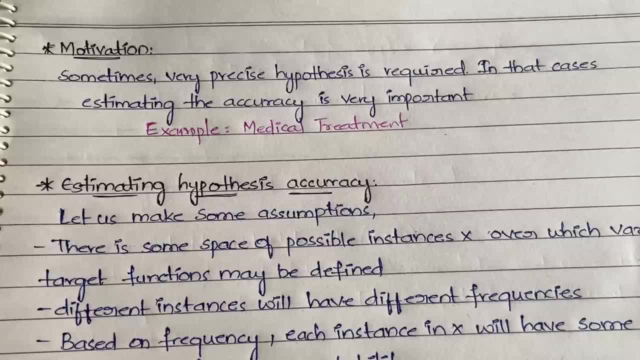 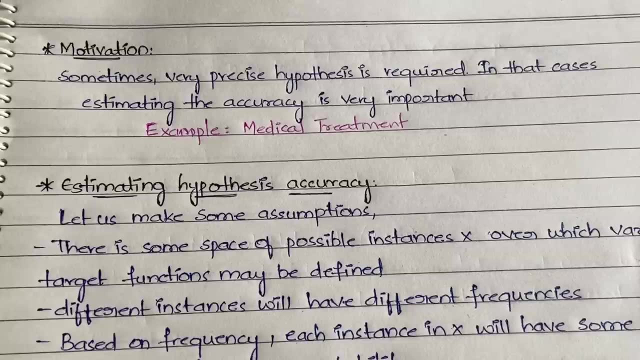 precise, very accurate hypothesis, then you have to estimate it, then you have to check for the accuracy because you want the best right, for example in medical treatments. so in medical treatments, what you do? you just randomly make a hypothesis after observing the patients reports, or something you don't make right, because if you make any, you know any hypothesis or any statement. 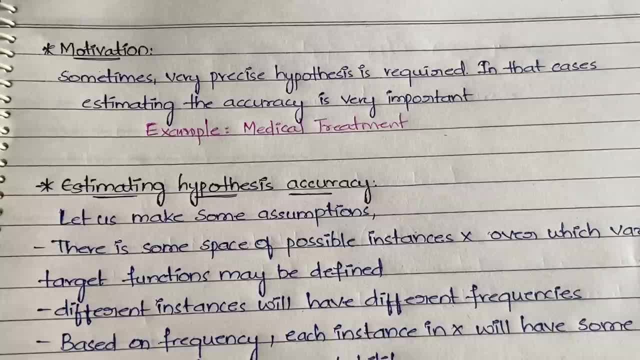 without proper knowledge, without proper studying, without proper experience or survey or whatever it is that will affect on the life of the patient, right? so whenever you are giving some suggestion to the patient, like you have to go through the so and so surgery or you have to go through so and so medicine, and all whenever you are, 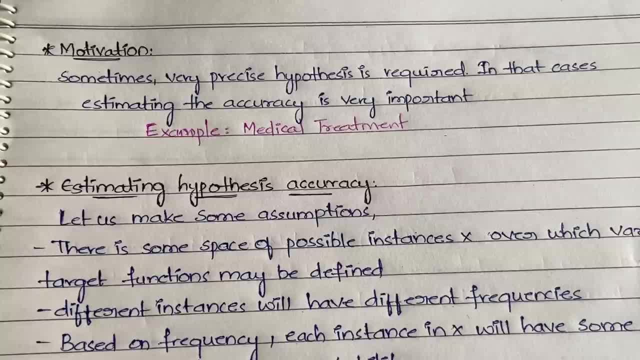 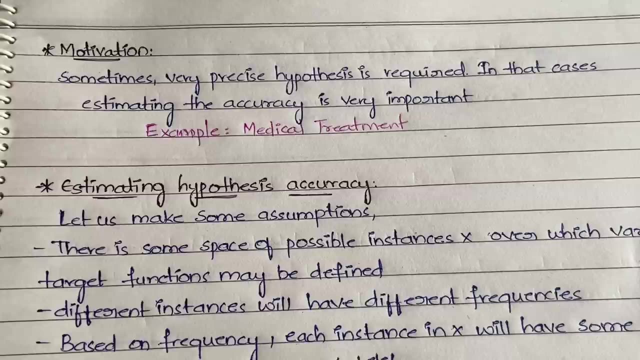 prescribing them, you should be very perfect, you should be very precise about them, right? because instead of you giving one medicine, if you are giving the other medicine for the patient- the patient, the problem the patient is having- that will not go right and instead it will show some side effects on the patient. so, whenever you, whenever there is a situation where you require, 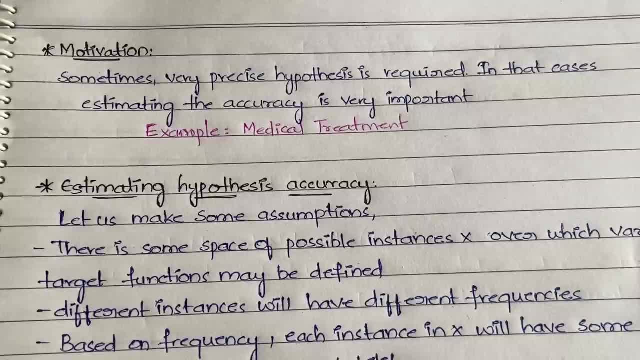 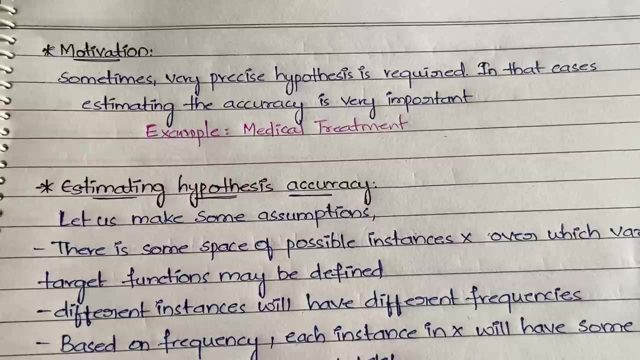 a precise hypothesis, then estimating the accuracy is very important so that you get the most accurate hypothesis. okay, done so. perfect example is in case of medical treatment. so whenever you are giving some suggestion or whenever you are giving some prescription, you should analyze the problem precisely. you should analyze the problem deeply. that means, whatever the solution you are giving, 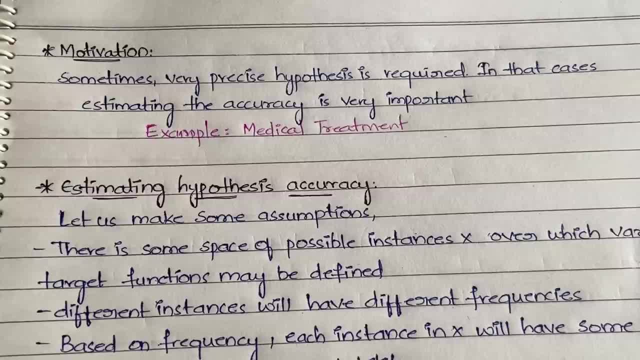 that should be maximum, accurate, right done. so that is why, if you go to a doctor, doctor will not just randomly give you a medicine or a prescription, but you should analyze the problem right first. he will ask you about your situation, about your health condition. he will check your. 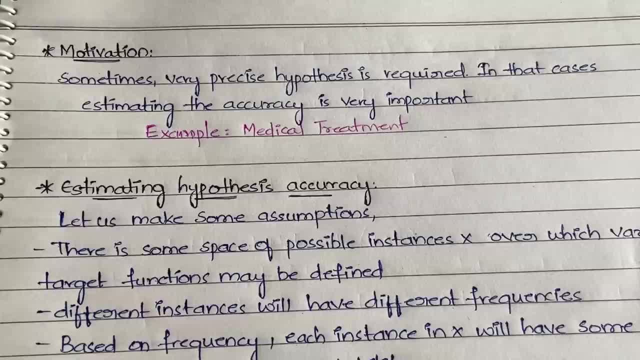 body temperature right. in some situations they'll check our blood pressure and even, in some situations, if they are not able to conclude anything, they will give us some reports, or, sorry, they'll ask us to take some tests, scans and all. then they will be prescribing. so they are very 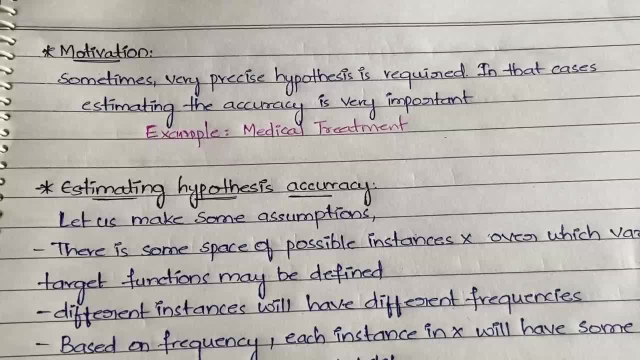 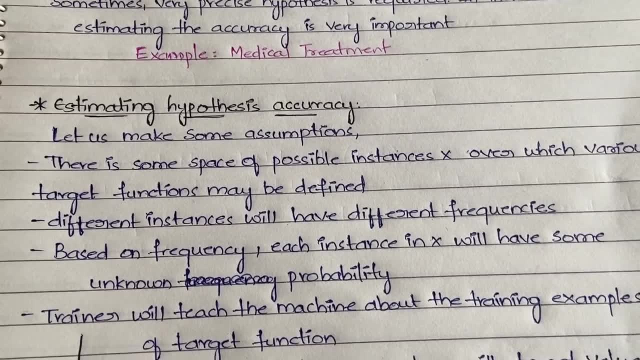 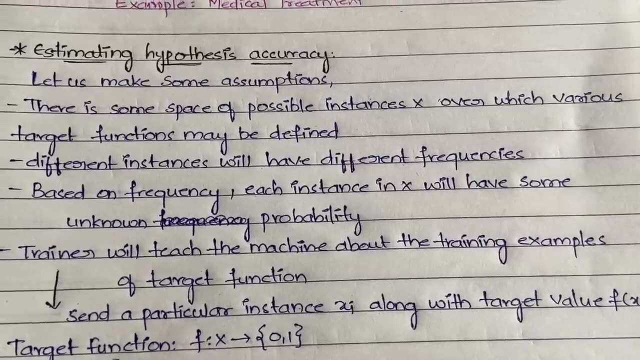 much particular about giving us a prescription, giving us a suggestion. so when, in these cases, we require very precise hypothesis, got it done so and what is the estimation, estimating hypothesis accuracy? so now let us see. how do we estimate the hypothesis accuracy actually? so first, before that, let us make some assumptions. so first let us consider. there is some. 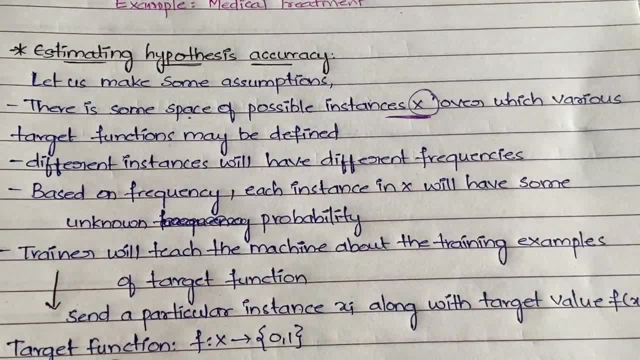 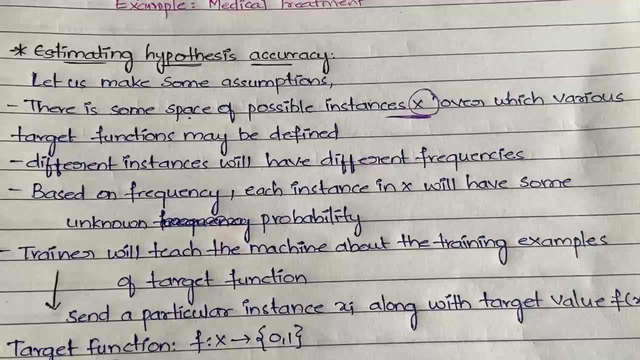 sample space of possible instances x. we are having x number of possible instances. okay, you know what possible instances are training examples and you know all those things. you know what possible instances are training examples. you know target function, you know training data, you know all. you know right training set and all so over which various possible instances are there. you know. 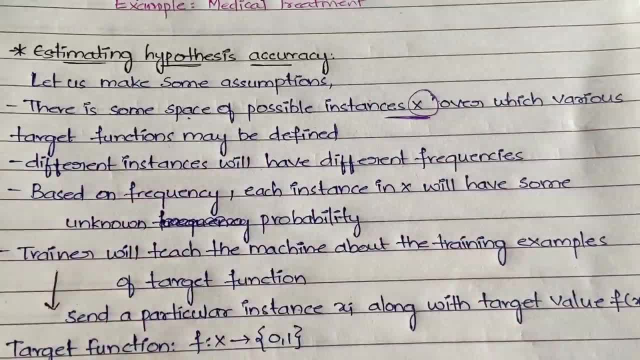 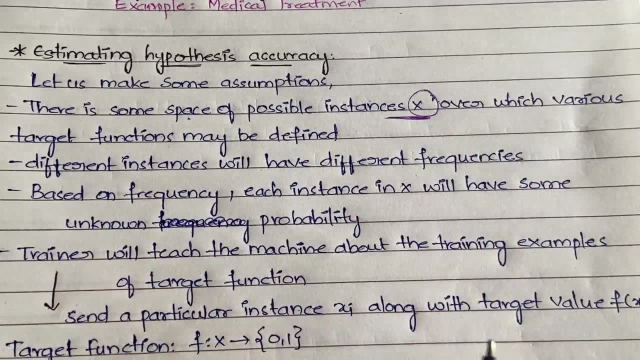 target functions may be defined. so, on these instances, you will be defining some target functions, right, and different instances will have different frequencies, right? so, for example, you are having a total of 100 instances in in x. you have total of 100 instances, right, and in that 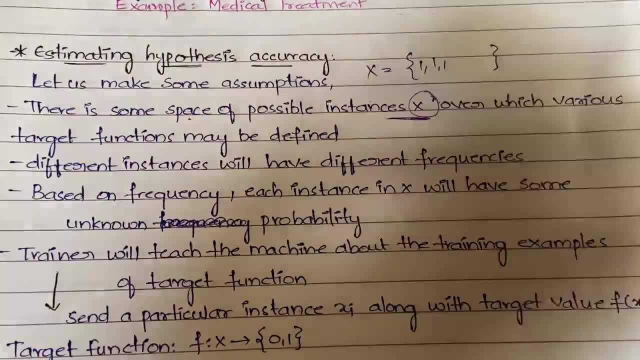 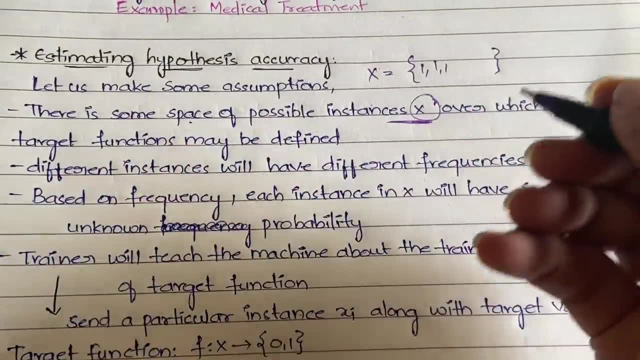 you have one one, one like that, or tall, tall, tall, head, head, head like that, you can have something based on the situation, right? so different instances will have different frequencies. suppose, let us take, we are rolling a die, right? so in the case of rolling a dice, what happens? 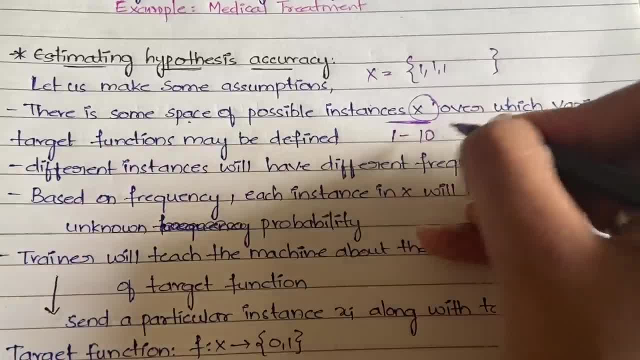 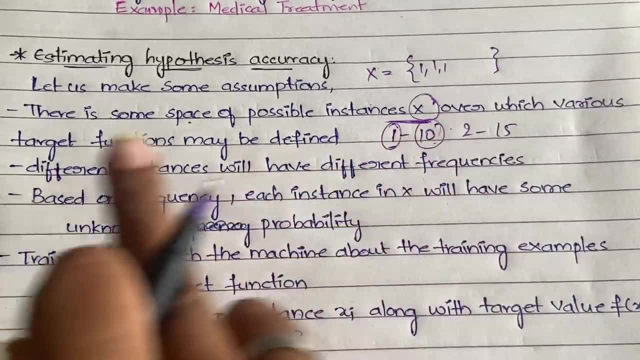 how many times you are getting one? suppose you are getting one for 10 times. you are getting two for 15 times. so what is the probability of sorry? what is the frequency of one here? 10, right, so each and every instance will have different frequencies. okay, so based on this frequency, you are going to 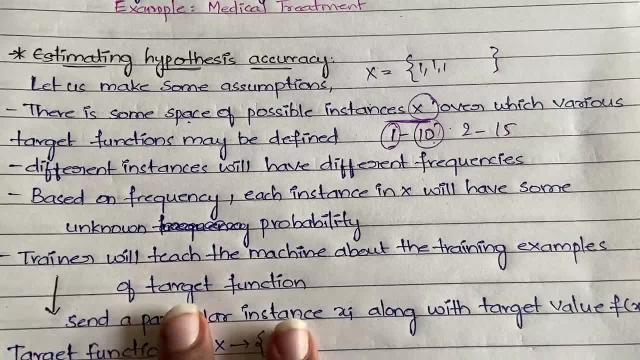 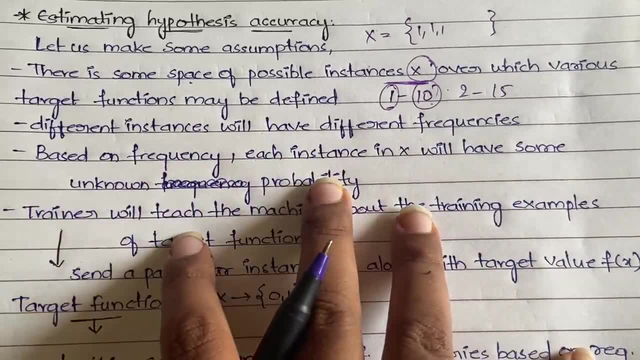 define an unknown probability. so the probability is unknown for us because, um, you know, we don't know what is the total sample size or some unknown probability we are going to define for each and every instance that we have took here. okay, done so once you define some unknown. 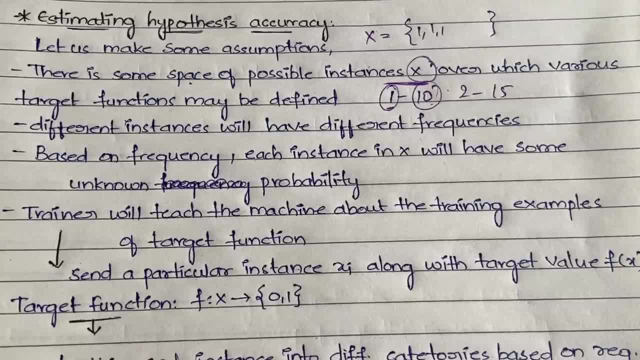 probability. what happened? what you have done till now? you have taken some sample, uh, in some possible instances x and for that instances you have defined some frequency and and based on that frequency you have defined some unknown probability. okay, done now. what trainer will do? what is the 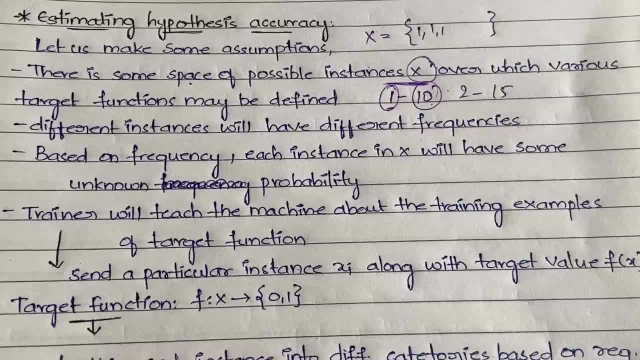 actual goal of trainer, trainer or a teacher. what they will do, they will teach students right. so in the same way, the trainer will teach the machine about the training examples of the target function. so what is the target function? what is the output that the machine has to give after learning? all these things? it will analyze, it will take some examples and the trainer 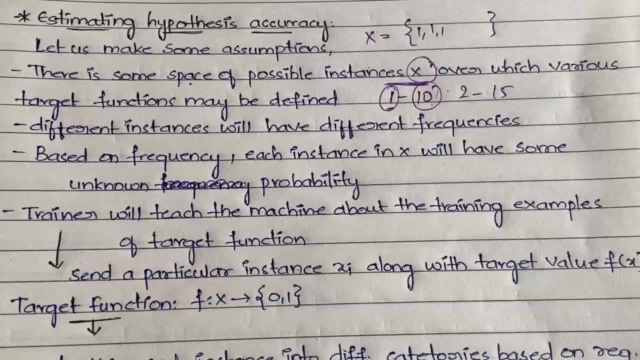 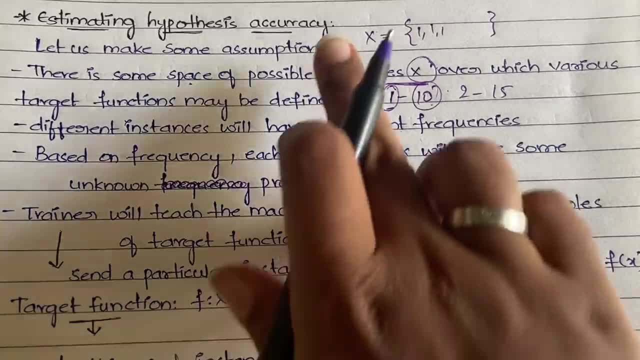 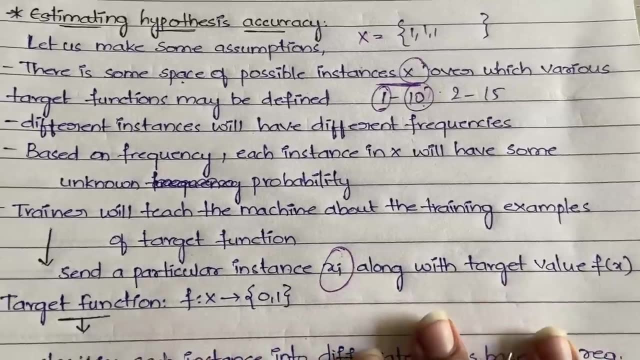 will teach the machine about that then. so how the trainer will teach? the trainer will send a particular instance xi. xi is nothing but one particular instance from set of instances. okay, so one particular instance, xi, along with the target value f of x, that is, along with the target. 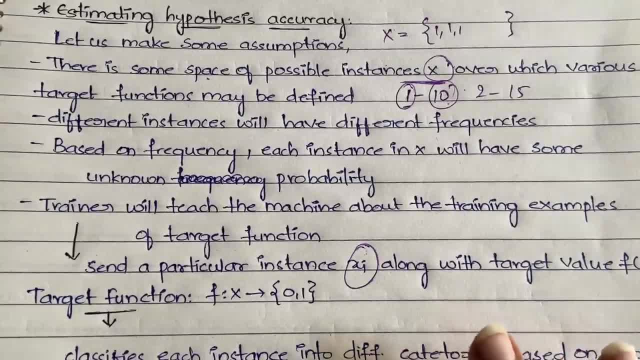 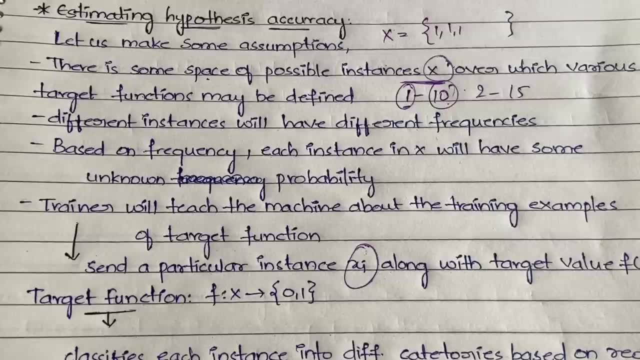 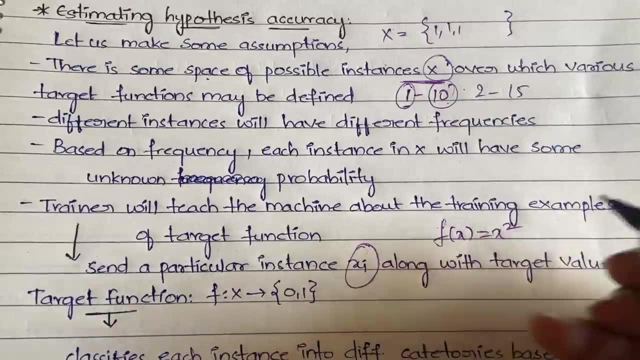 function f of x, the trainer will send an instance to the machine so that the machine will learn based on the target function. so based on the target function, according to the value of xi, it will generate the output. suppose the target function is f of x is equal to x square. okay, then xi? we are giving xi as 2. then what happens actually? 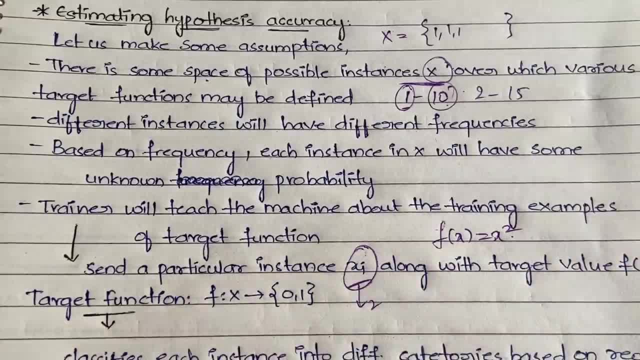 what is the target function? x squared so 2 square 4, 4 would be the output, like that. so it will send the instance and also target function and so that the machine will perform according to the target and give the output. okay, done now. the target function, uh, is like randomly. it is defined as f of